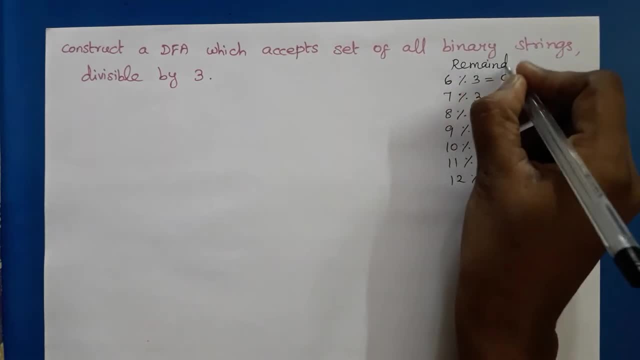 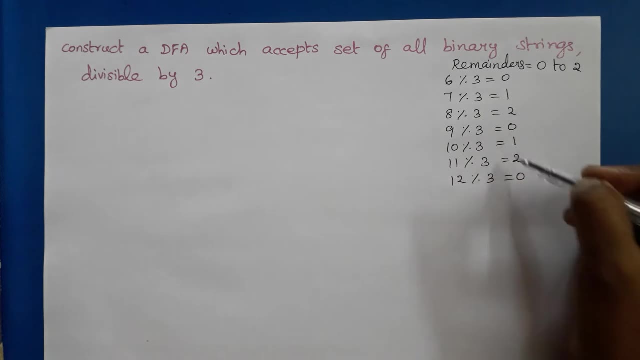 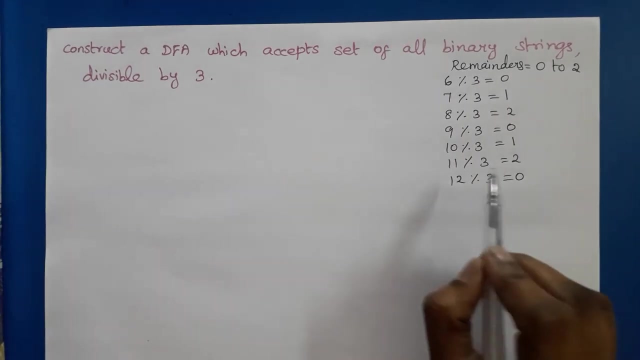 always get the reminders from 0 to 2, 0 to divisor minus 1, so 0, 1, 2, 0, 1, 2. so it is going on. so to construct a DFA we need three states: one to represent the remainder 0, another one is remainder 1, another one is remainder 2, so we are. 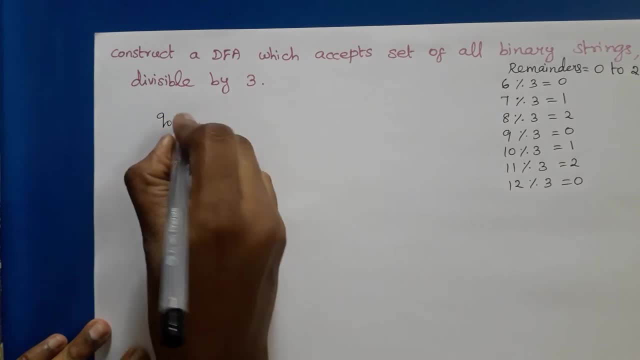 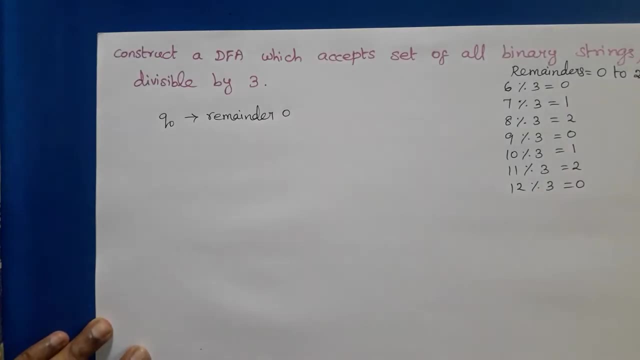 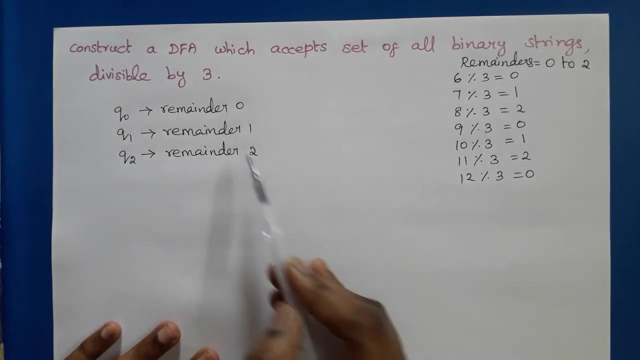 going to use three states. so Q naught for representing remainder 0, Q 1 for representing remainder 1, Q 2 for representing remainder 2, because we will get only three reminders: 0, 1, 2. and whenever we get the remainder 0, we can. 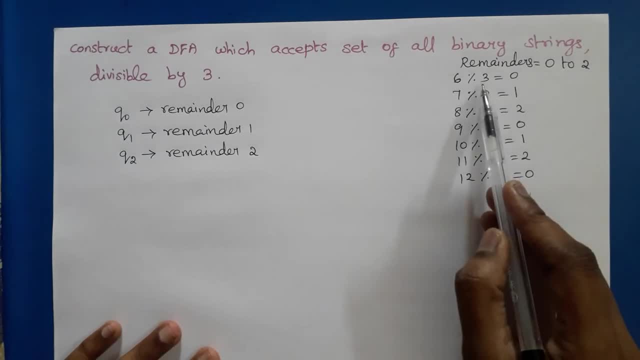 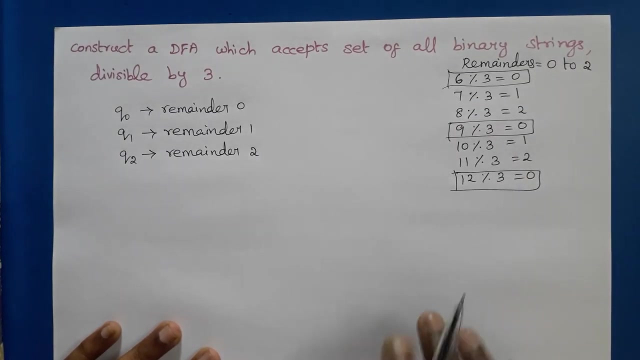 say that the number is divisible by 3, since 6 is divisible by 3 because we are getting number remainder 0.. Similarly, 9 is divided by 3, 12 is divided by 3, so whenever we get the remainder 0, we can say that that number is divided by 3, so we can make Q naught. 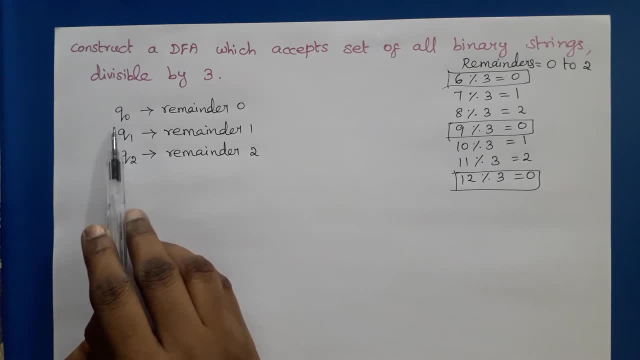 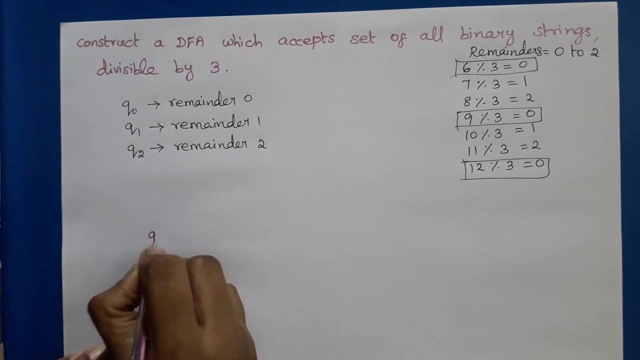 as a final state, because Q naught represents the number divisible by 3. so in this problem Q naught is start state as well as final states. Q 1 is representing remainder 1, Q 2 for remainder 2. now we can construct a DFA. Q naught is start state as well as final state, and this is a binary number. 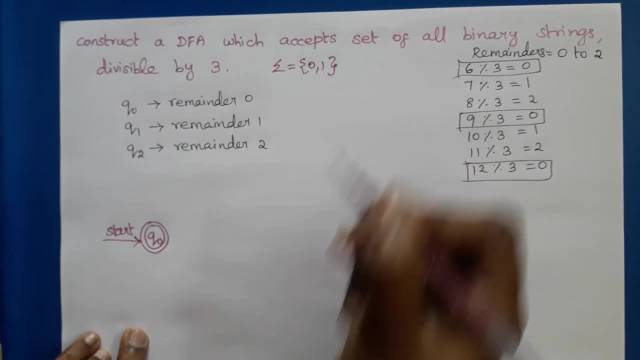 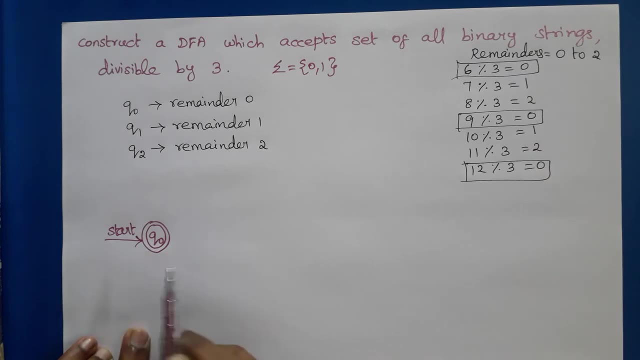 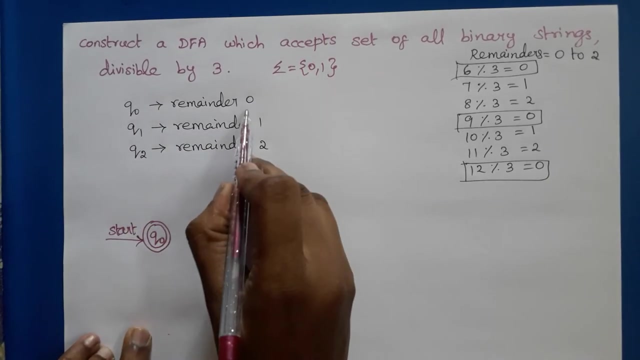 binary string, so sigma is 0 and 1 input alphabet. so from each state we have to construct transitions for 0 and 1. so in q naught, if the next input is 0, next input is 0 means the remainder is 0, only 0. mod 3 is 0, so remainder 0 means we need to draw the. 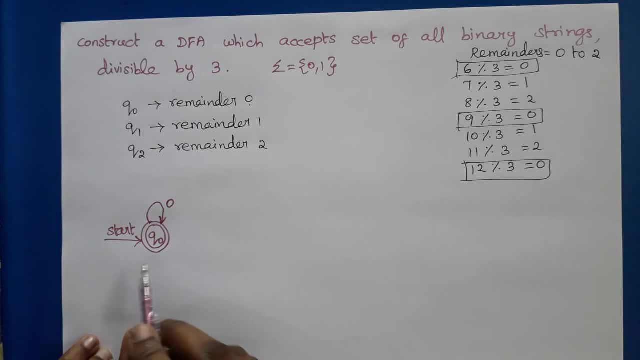 the transition for state q naught, then from q naught the input 1, input 1. 1 means 1 divided by 3, 1 modulus 3 will give 1, remainder 1, so it goes to q1. so from q naught 1 goes to q1, because we 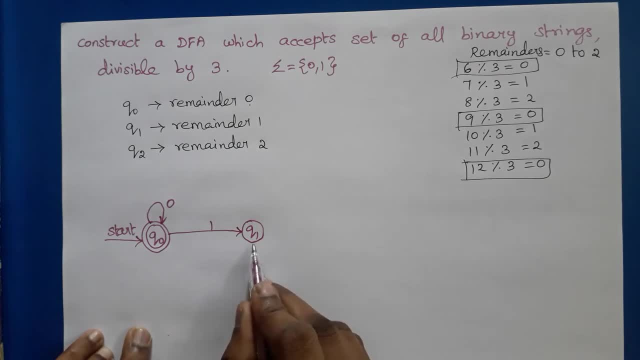 will get the remainder 1 now in q1. now we have to consider the current state q1 so we can reach state q1 after reading 1 only. so after reading 1, the next input is 0. assume that the next input is 0. so the decimal equivalent for 1, 0 is 2. so when we perform odd operation for this 2. 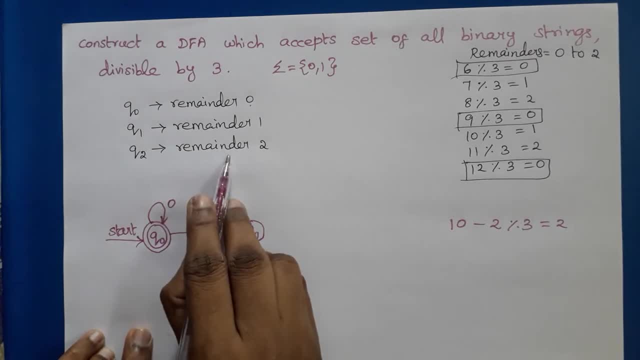 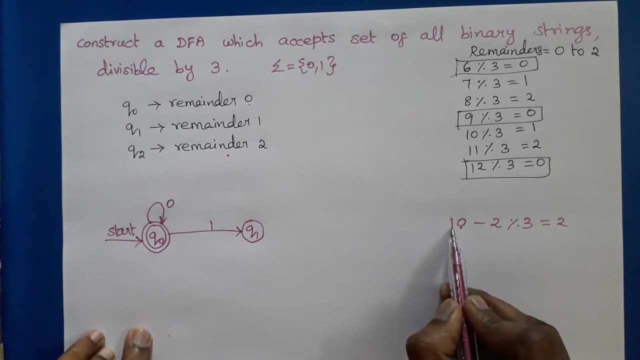 we will get the remainder 2, so remainder 2 means it should go to q2. so in q1, if the next input is 0, we have already recognized, we have already read 1. so the next input is 0 means 0, it is 2. so 2 mod 3 will give the remainder 2, so it should go to q2. 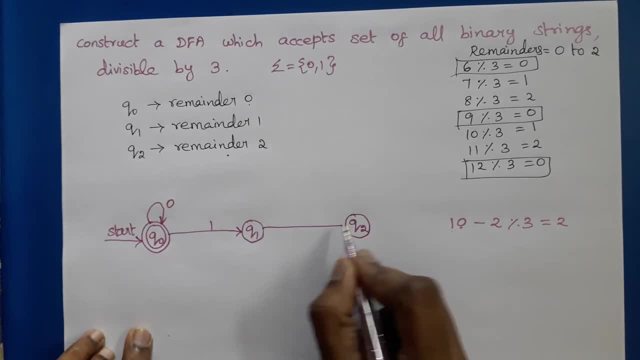 so from q1, 0 goes to q2. similarly, we need to consider 1 from q1, so we have already seen 1. now the next input is 1, so the decimal equivalent is 3. 3 mod 3 is 0, so it should. 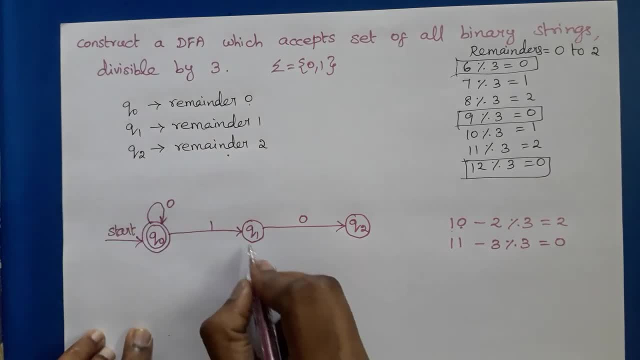 go to remainder 0. remainder 0 means it should go to q- naught. so from q1, the input 1 means it should go to q- naught. then we need to consider q2. so from q2, 0 is the next input, so q2 can be reached. 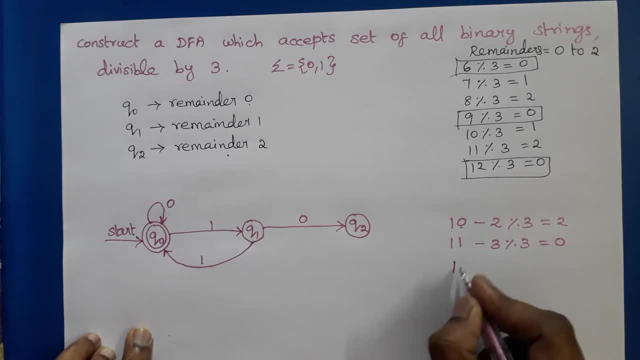 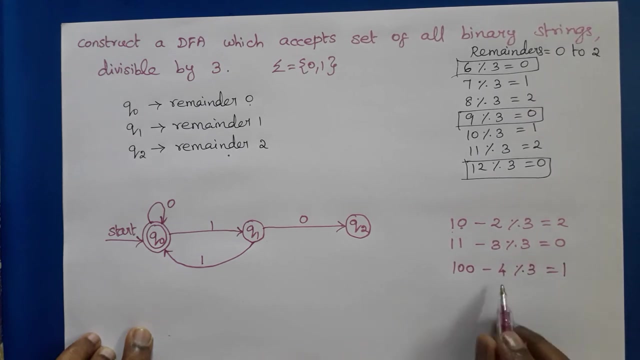 after recognizing, after reading: 1: 0. 1, 0 is already. we have read, so the next input is 0, so the decimal equivalent for this number is 4. 4 mod 3 is 1, so remainder 1. it gives remainder 1, so from q2. 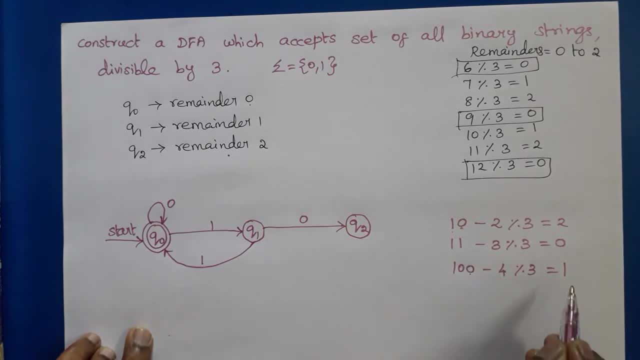 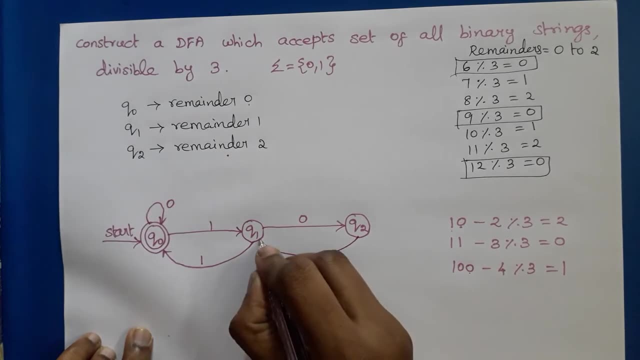 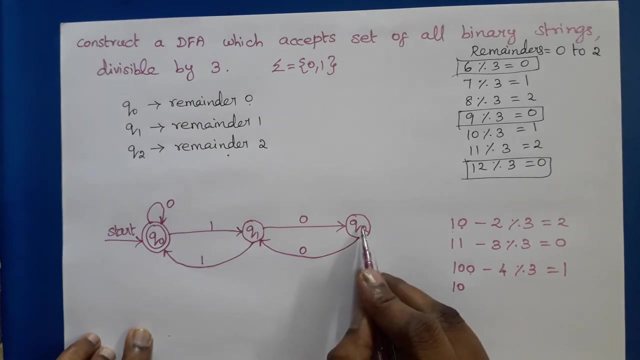 if 0 is the next input, then definitely it should give the. it gives the remainder 1, so remainder 1 means then it should go to q1, so input 0 goes to q1. similarly, after reading 1: 0 in q2, if the next input is 1, so it is 5. 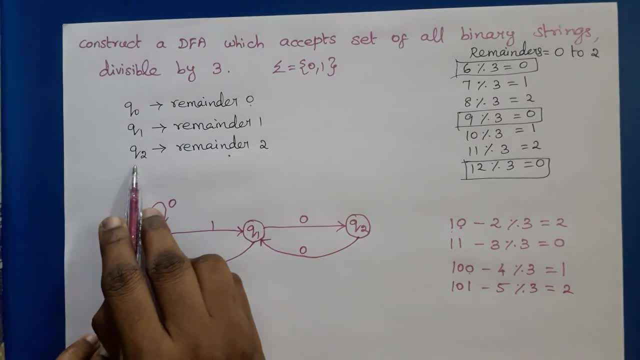 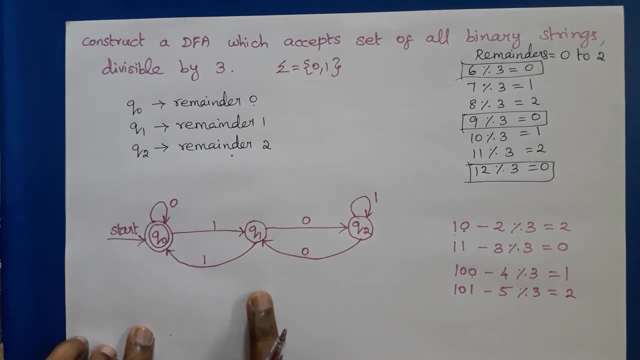 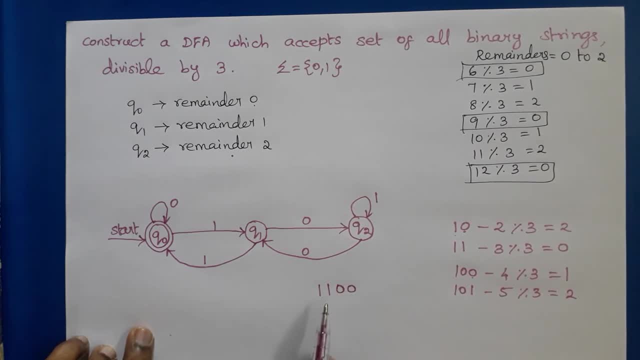 string is divisible by 3. so we can check whether a binary string is divisible by 3. so we can check 1 1 0, 0. now we have to check whether this input string is accepted by our dfa. this is the number divisible by 3, binary string divisible by 3. so definitely it should be accepted by our dfa. so 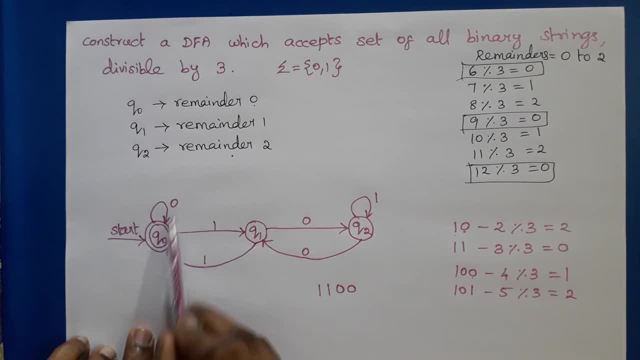 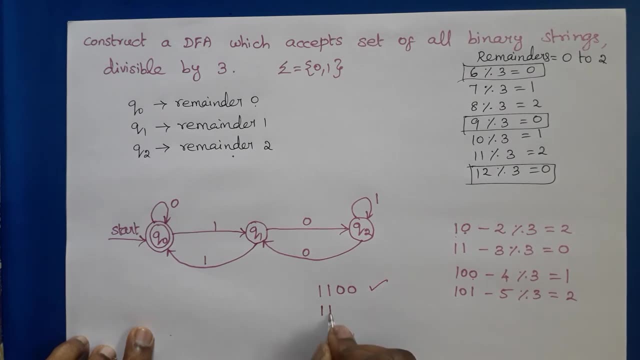 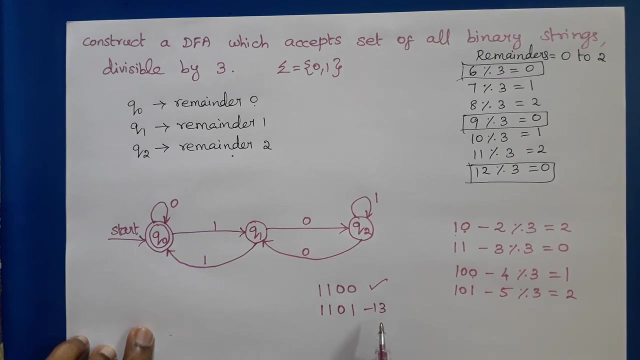 now we can check it: 1 1 0, 0, so it is accepted by our dfa. similarly, we can consider a binary string: 1 1 0, 1, so this is the decimal equivalent 13, so it is not divisible by 3, so definitely. 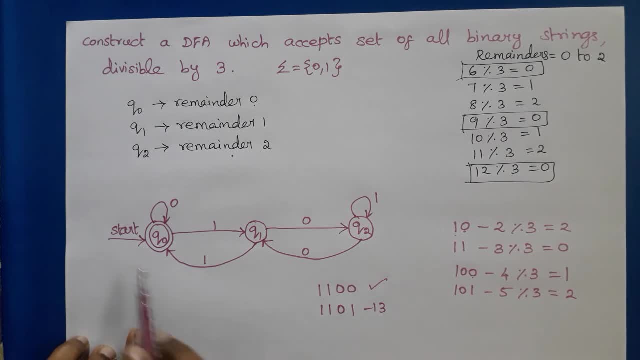 it should not reach the final state, so 1 1 0, 1. it is ending with q1. q1 is not a final state, so it is rejected by our dfa and when we divide this number by 3, we will get the remainder. 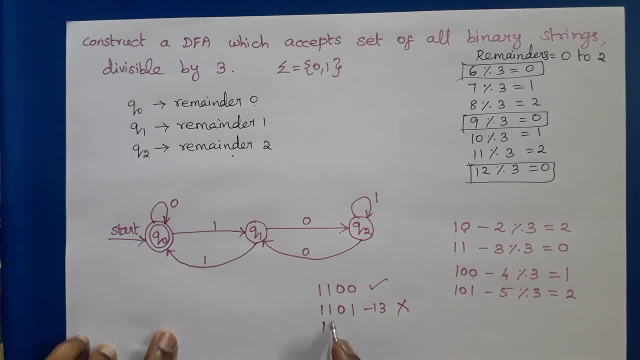 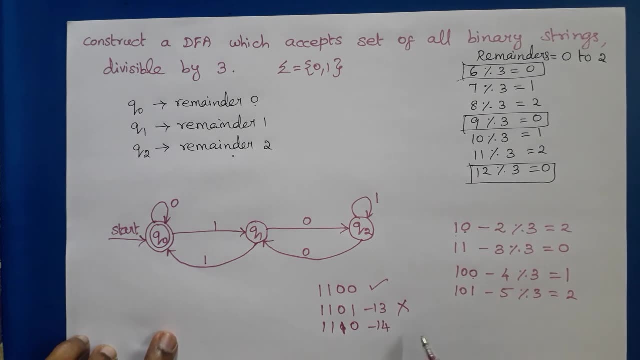 1, so we are ending with 1. similarly, if you consider 14, 14 means 1 1 0, 1. so this is the decimal equivalent, 13. so it is not divisible by 3, so definitely it should 1 1 0. so when we divide this number by 3, we will get the remainder 2, so we will end with q2. q2 is: 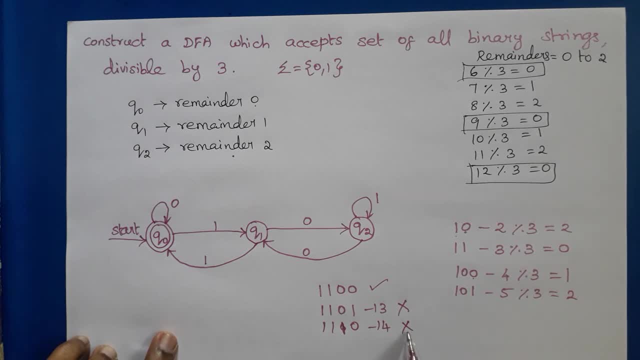 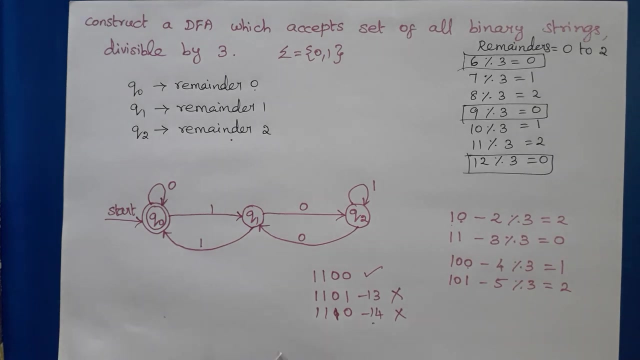 also not a final state, so it is also. it should also be rejected by our dfa. so 1 1 1 0, 1 1 1 0. we will end up with q2 and it is also rejected by our dfa, so we can construct a binary strings. 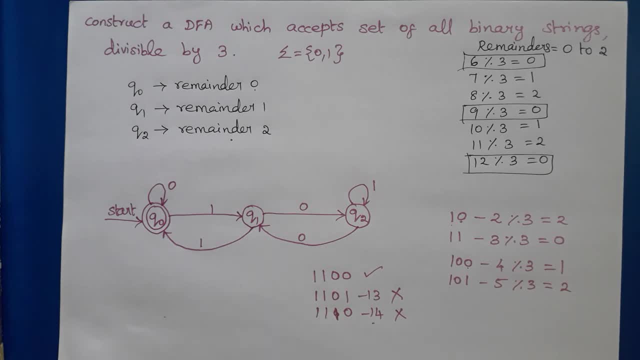 divisible by 4: 5 also in this similar way. thank you, thank you.